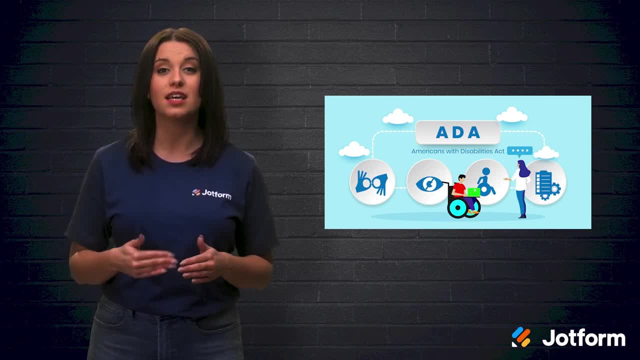 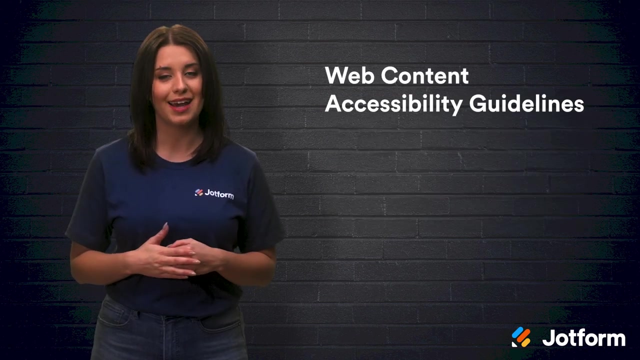 technology, but no guidelines were really put into place addressing accessibility within technology. That's simply because the ADA was enacted before the internet became as extensive as it is now. So to address this gap, the World Wide Web Consortium created the first Web Content Accessibility Guidelines in 1999.. 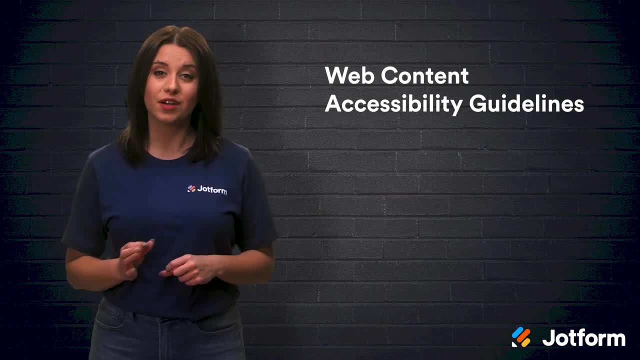 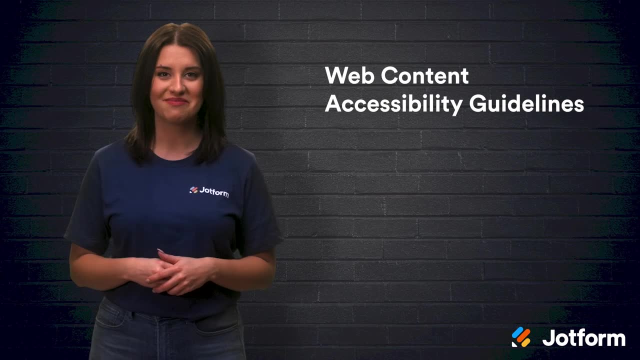 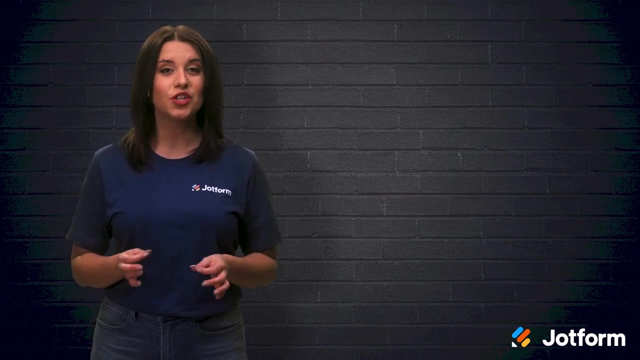 The guidelines name four principles to make web content more accessible to people with disabilities and three levels of conformity which determine an organization's performance in each area. Let's discuss the four principles and levels of conformance. The four principles of accessibility are actually known as the POUR principles. 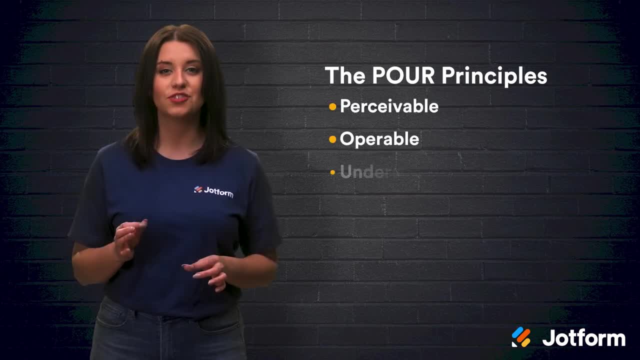 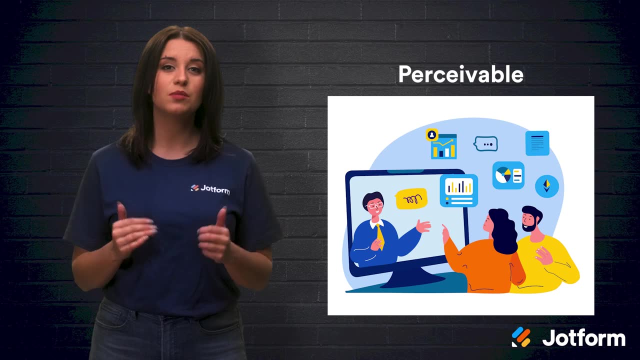 This acronym stands for Perceivable, Operable, Understandable and Robust. First Perceivable: This means that anyone viewing the page should be able to consume all information through a variety of senses. No aspect can be invisible to users. There should. 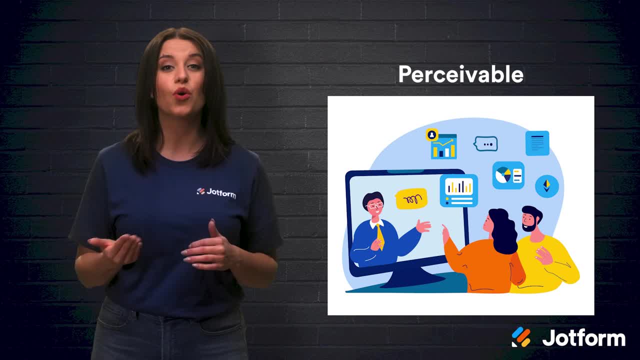 be text alternatives for non-text content and captions or audio descriptions on multimedia. There should also be an option to view the content in a different way by enlarging the font, reading it aloud or changing the text color. Everything on the page must be visible to anyone. 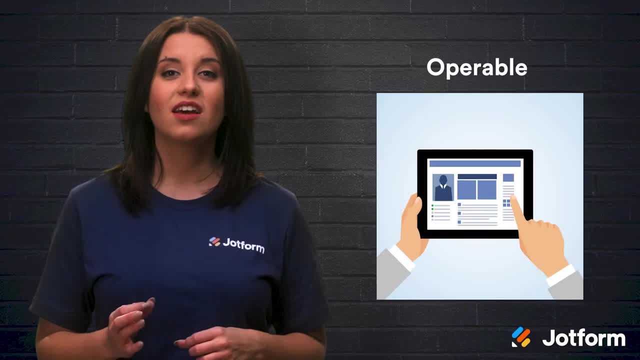 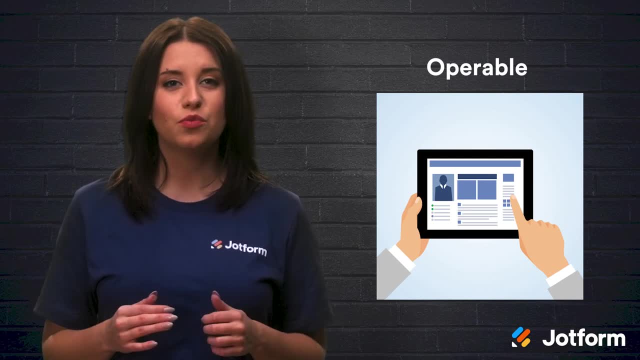 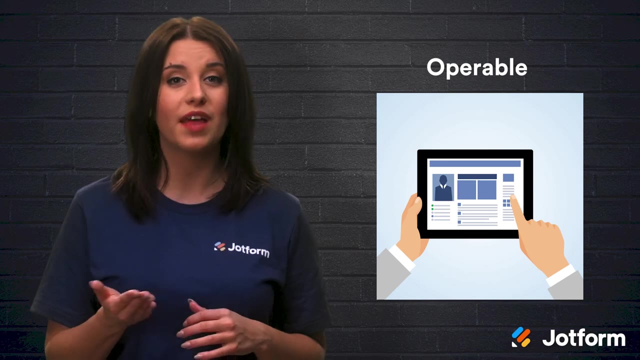 who wants to view it. Second, Operable. The content should be navigable for people who don't use a mouse and keyboard to access the web. Any specialized tools should be able to navigate the content. In this case, Operable also means users can view the content at their own speed without 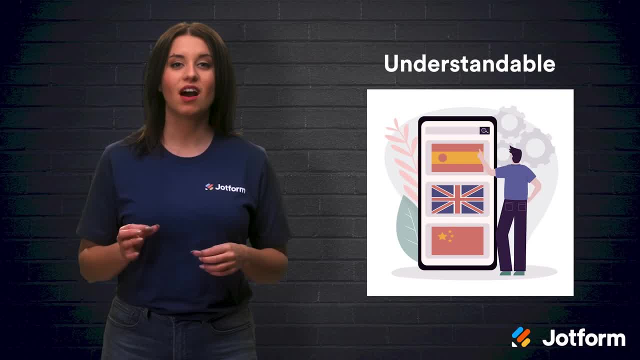 any time restraints. Third is Understandable. Content needs to be understandable in order to be accessible. If certain visitors can't comprehend your content, then it isn't accessible to everyone. This means you need to identify what language the text is being presented in. 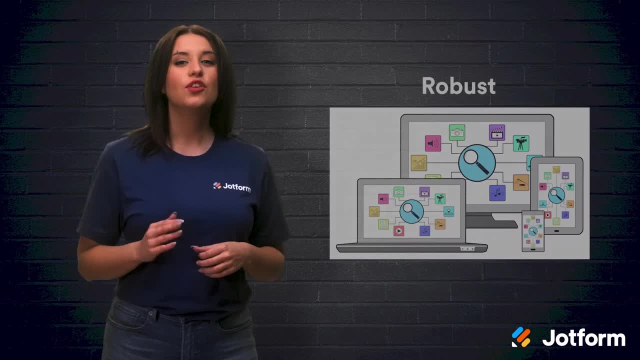 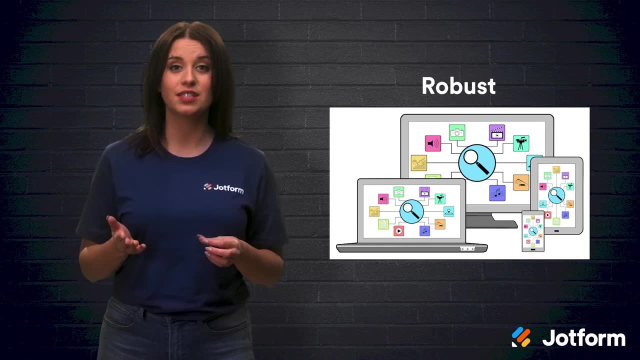 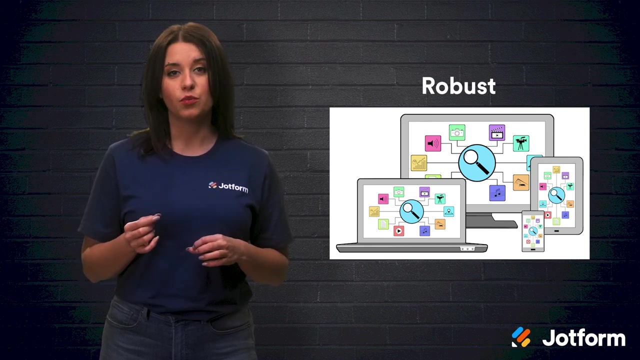 and give the content at an appropriate reading level. The fourth and final principle is Robust. Robust content is available on multiple devices, including computers, tablets and mobile devices. Your interface should also be compatible with different assistive technologies like screen readers. Now let's go into the three levels of conformance. 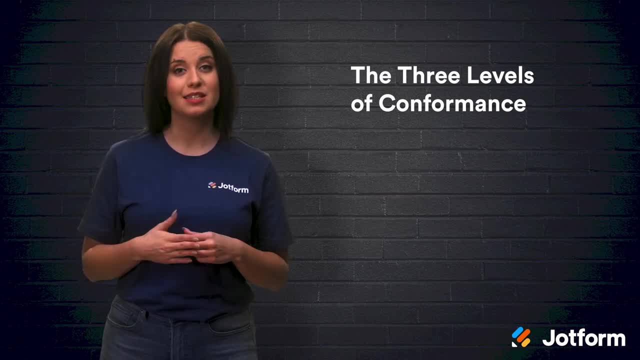 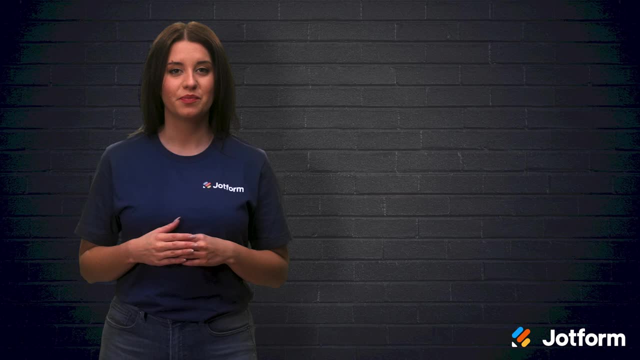 These levels are what determine how accessible your website really is. If your website meets the expectations of a certain level, then your website has conformed to that specific level. The first level is called Level A. This is the beginner level and at the most basic level. 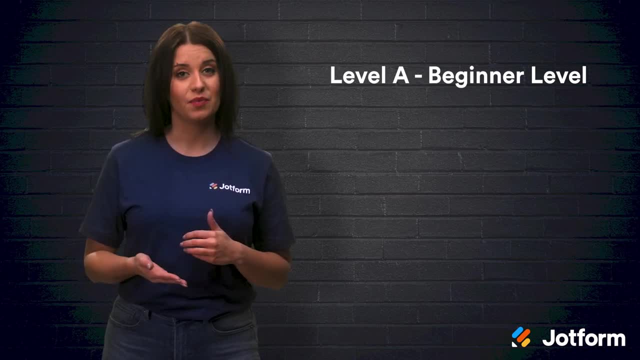 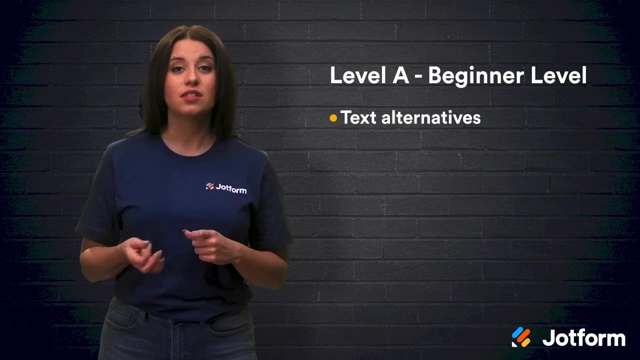 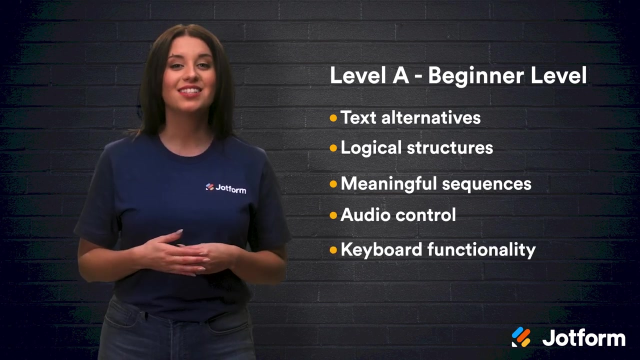 all websites are expected to meet the criteria within Level A. Conforming with Level A means that your website has the simplest features of accessibility implemented. This includes text alternatives, logical structures, meaningful sequences, audio control and keyboard functionality. This is the first step to making your website accessible. 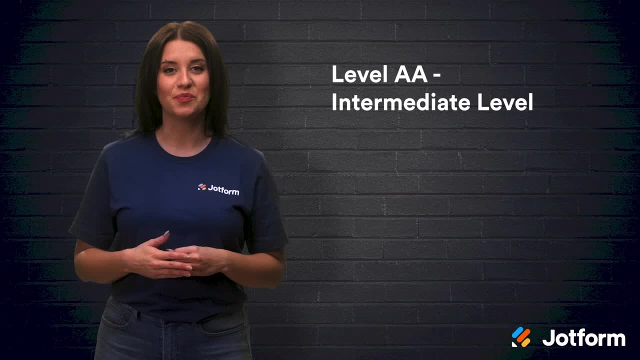 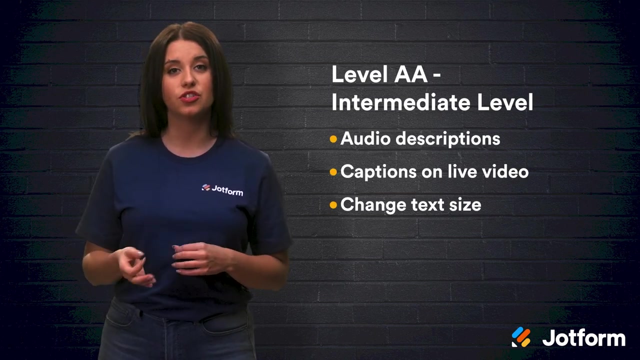 The second level is Level AA, or the intermediate level. Criteria from Level A must already be met in order to move up to Level AA. This level requires more advanced aspects to accessibility, including audio descriptions, captions on live videos and the ability to change the size of the. 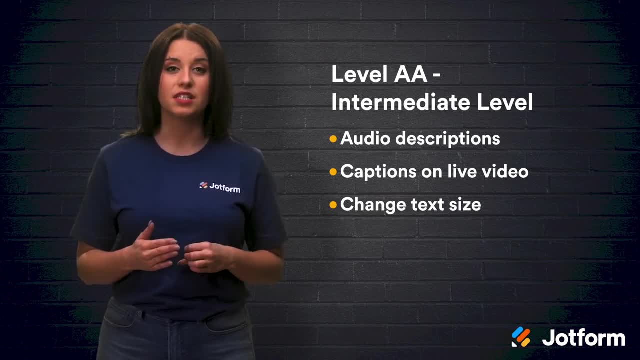 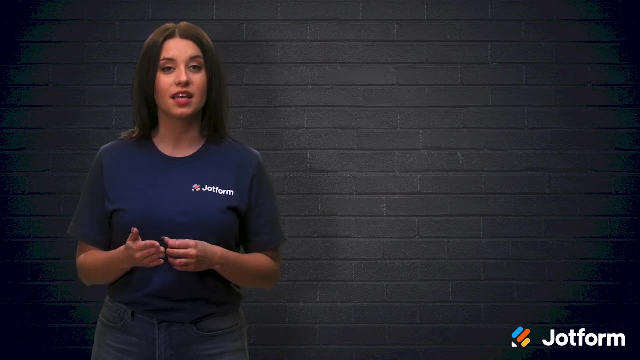 text. According to Glenn Schubert, the Executive Vice President of Marketing at BrailleWorks, this level achieves reasonable accommodation so the users can access all content and easily navigate the site. In fact, Level AA is the default for most organizations- Any websites that comply with. 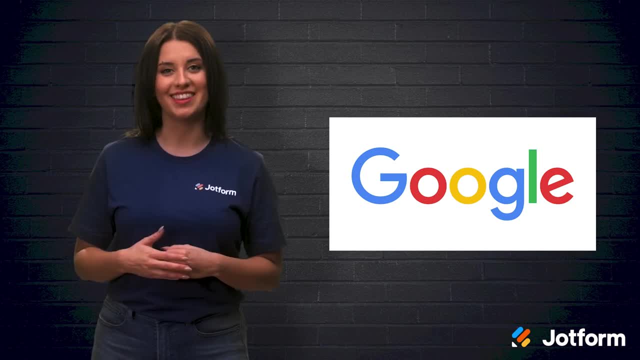 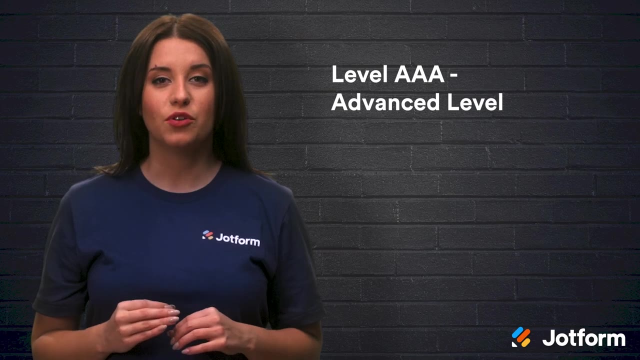 Google's best practices have already met several of the criteria at this level. There's a lot of overlap between Level AA and Google's best practices, like using clear heading and labels on your website, And the final level is considered Advanced Level- AAA- In order to reach this level. 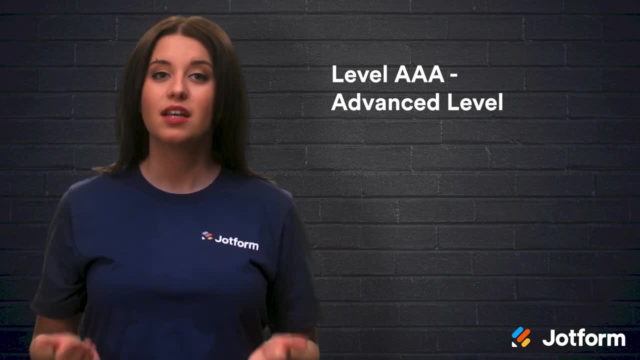 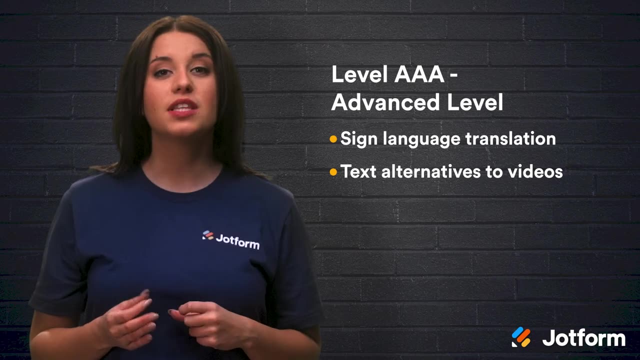 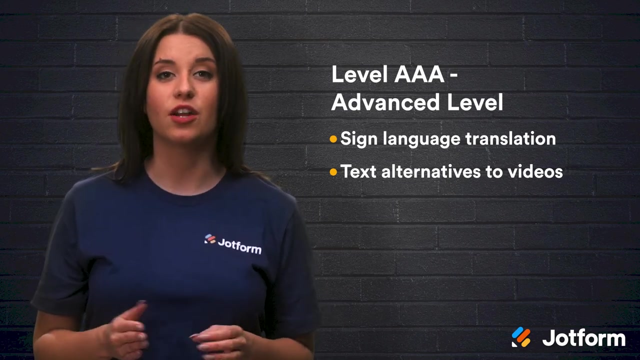 your website has to meet the criteria from the previous two levels. Some criteria for Level AAA include sign language, translation and text alternatives to videos. Features like these are great, but they aren't always doable. Glenn Schubert says that there are some additional standards in AAA that are very 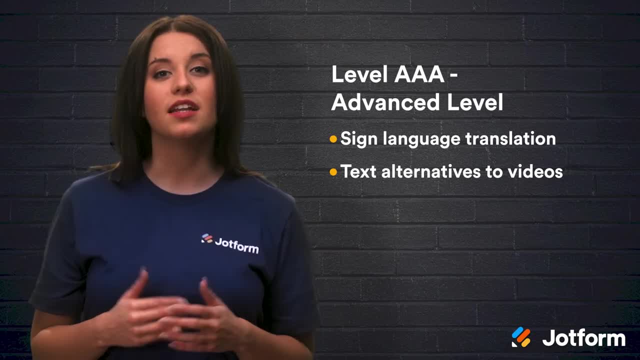 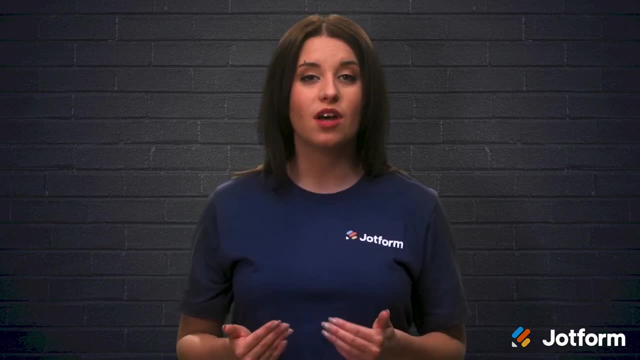 labor-intensive and very cost-prohibitive. This means that not all websites can satisfy every requirement. If you're looking for an accessible online form builder, jotformcom is the place to go. We offer form templates that are complete, customizable and easy for anybody to use.